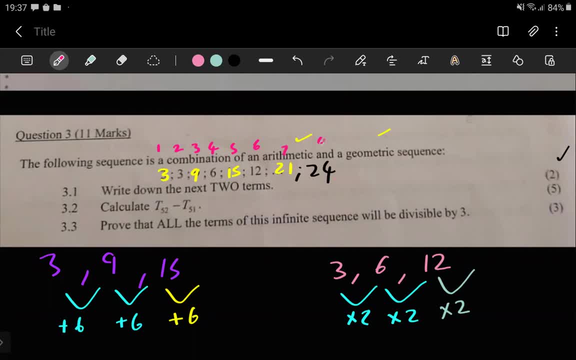 five, six, seven, eight, going on and on and on. So somewhere along the lines, you're going to have T51 and you're going to have T52.. We don't know what T51 is, we don't know what T52 is, but then they want us to take T52 and subtract T51. 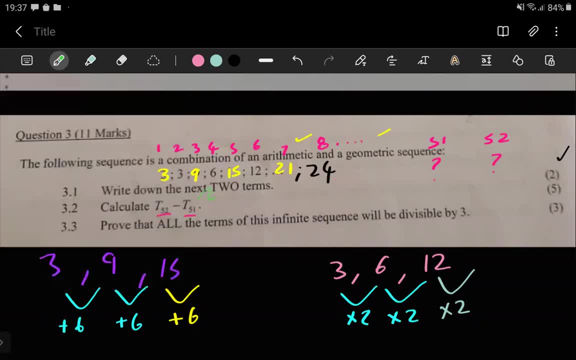 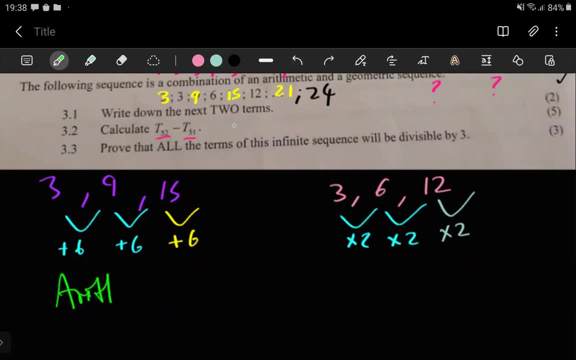 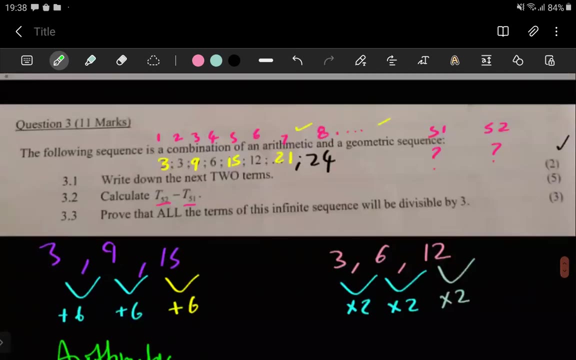 So already just by looking at how our equation is set up, right, you can already see that. looking at the arithmetic sequence- let me make sure this is clear- This is the arithmetic Arithmetic. Looking at the arithmetic sequence: right, it is clearly in the arithmetic sequence takes. 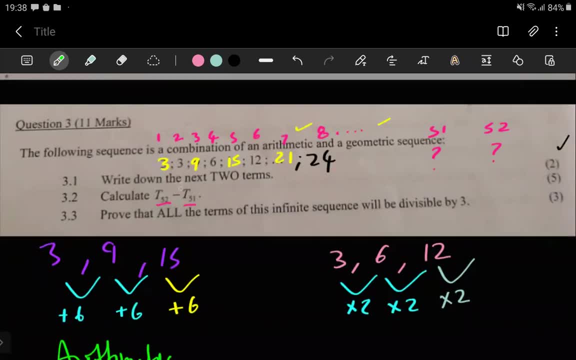 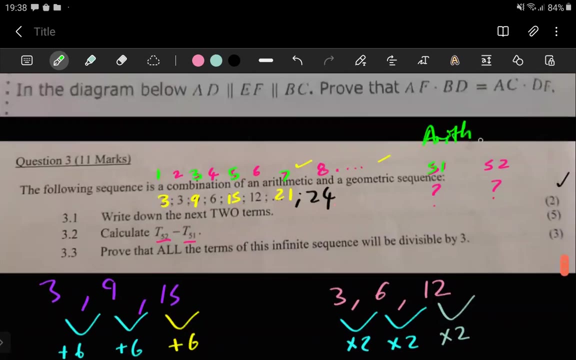 is basically in the positions that are odd. You see position number one, position number three, position number five, position number seven. So automatically, position number 51 is going to come out from the arithmetic sequence And then the rest of the term. 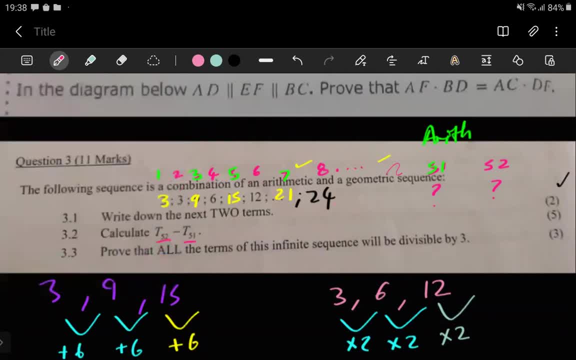 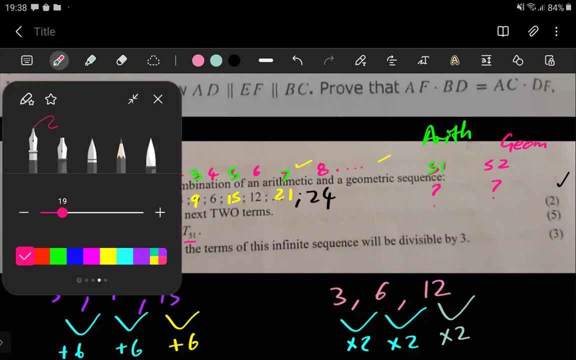 which are in position number two or six, going on to like 52. Those ones are going to be part of the geometric sequence, you see. So let's just put here This one is going to be is going to come out from the geometric sequence. So what we just need to now do, which is not going to be too crazy, is we just need to think to ourselves: okay, fine, from these two sequences, 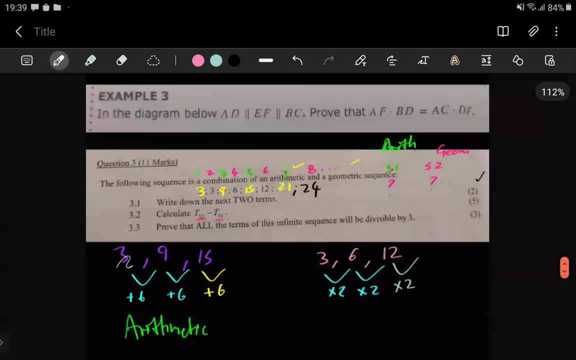 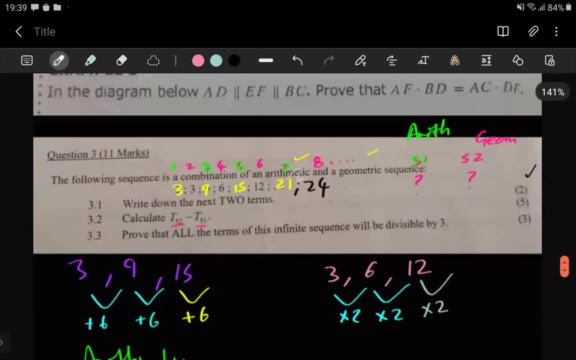 individually right. we're clearly seeing that term number one, term number two, term number three going on and on and on. We need to see how we can link it to this original one, you see, of which that's not going to be too difficult. 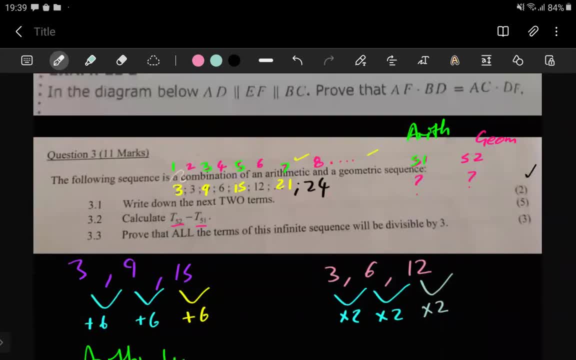 And here's why You can already see that every second term here is from the geometric sequence. That's one thing we can already see. Every second term here is from the geometric sequence. Okay, So looking at the geometric sequence, I mean 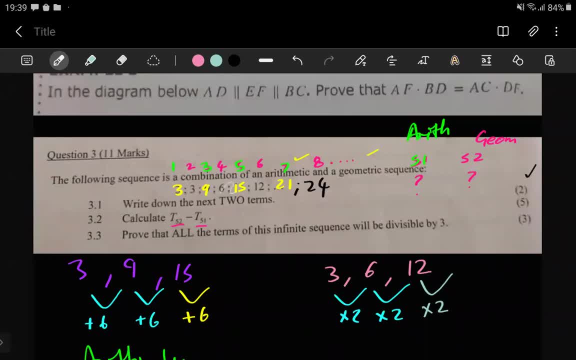 something that's in position number 52, for the original sequence is technically going to be in position 26,. if you're just considering the geometric sequence alone, you see, because, look at it, This is in position number one. or the geometric sequence, This is in position number two. This is in position number three. this is in position number four. 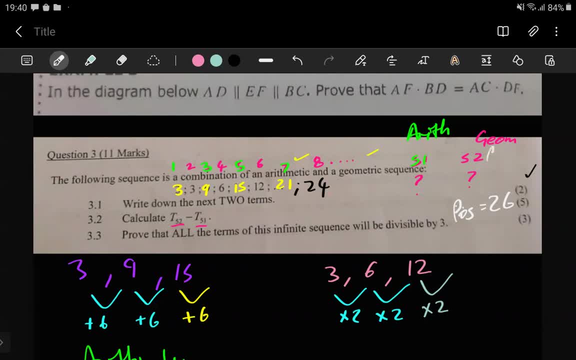 So obviously this is going to be the geometric sequence here. this would be in position number 26.. You can even just look at how the trend is going. This is in two right, But it's at position number one. This is in four, but it's in position number two. This: 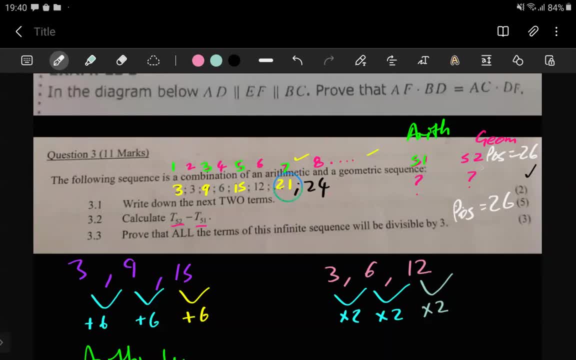 is in six, but it's in position number three, going on and on and on. So this is going to be in position 52 for the original sequence, but it is actually position number 26 for the geometric sequence And that same analogy. you want to use it for the arithmetic sequence. It's going to be. 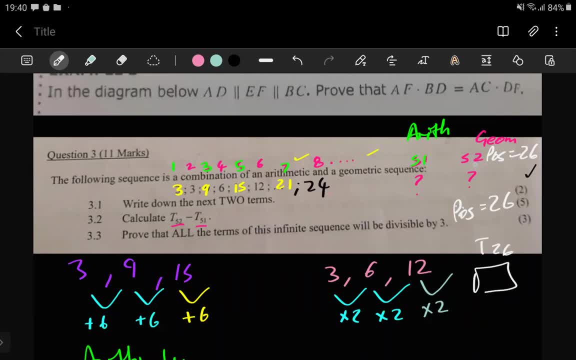 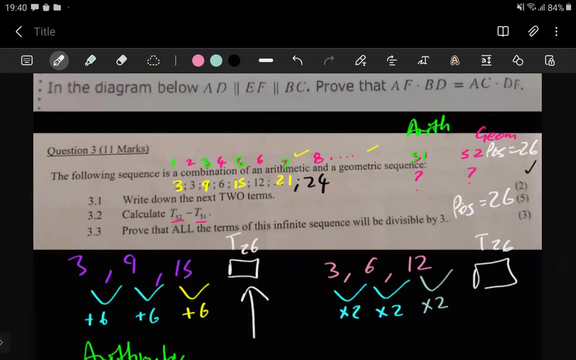 the exact same thing, because these are 52 values in total, but then the ones that make up the arithmetic sequence. it is just going to be 26 as well. So already you know that somewhere here there's something in position number 26.. So what is in position number 26 for the arithmetic? 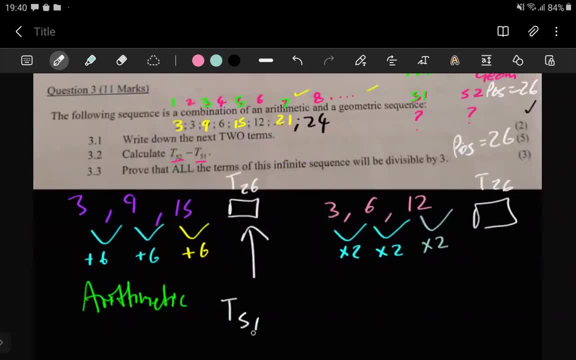 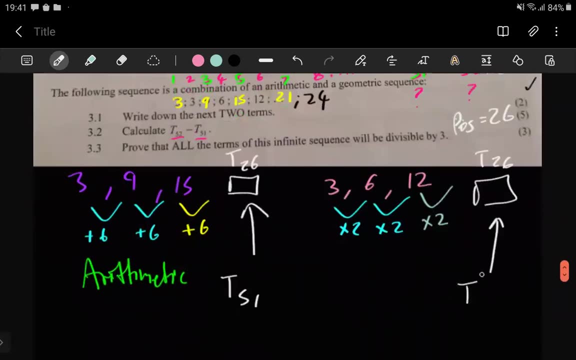 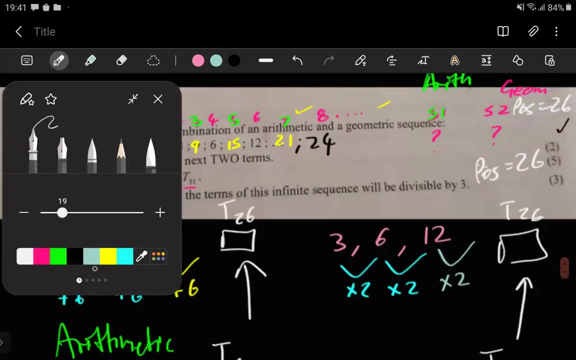 sequence: here this is what's in position 51 for the original one, What's in position 26 for the geometric. here this is what's in position 52 for the original one. So, without making too much of a mess of this question, right, All we? 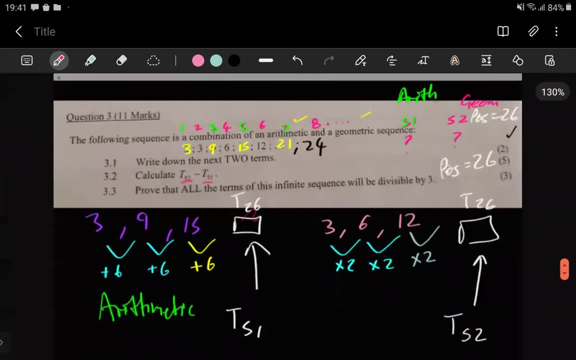 have to do is, for this arithmetic sequence, let's work out what's in position 26,. get that answer. For this geometric sequence, let's also work out what is in position 26,. get that answer, And then those two answers will represent what should go here and what should go. 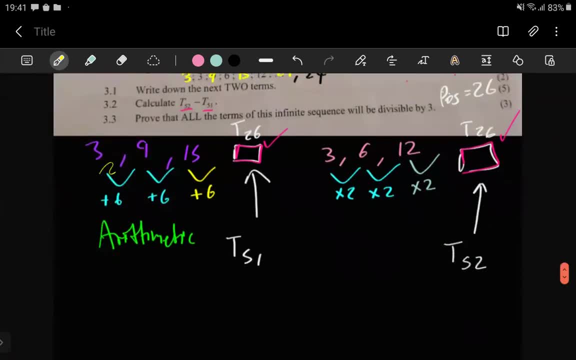 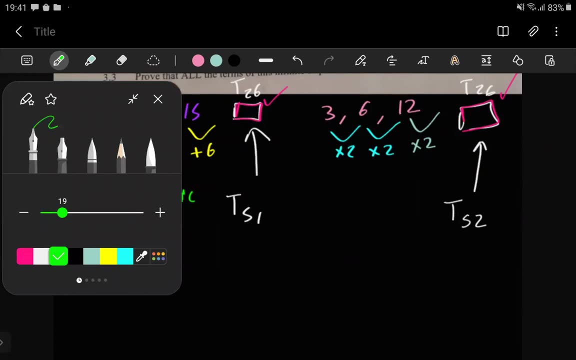 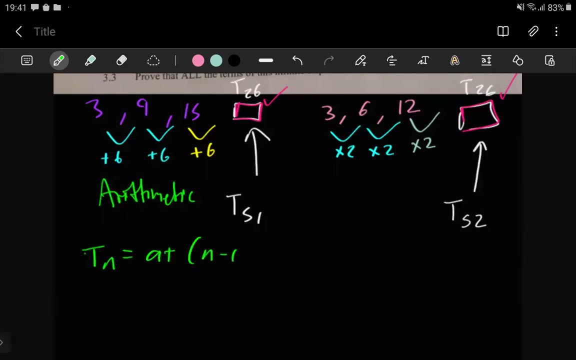 over there. So let us do it So here. this is just an arithmetic sequence. We know that to get something in position 26, we just have to use the general term tn. it's got a plus n, minus 1d. So a here is 3,, n is 26.. And then d. what is d? D is a common. 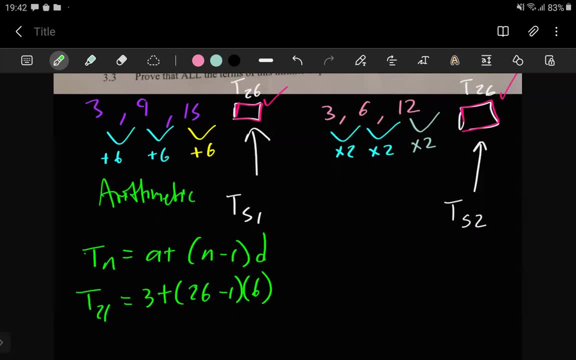 difference right, which is a 6.. There we go. So that's what we're going to do for the arithmetic, For the geometric. we do the same, but we do the same for the geometric, We do the same for the. 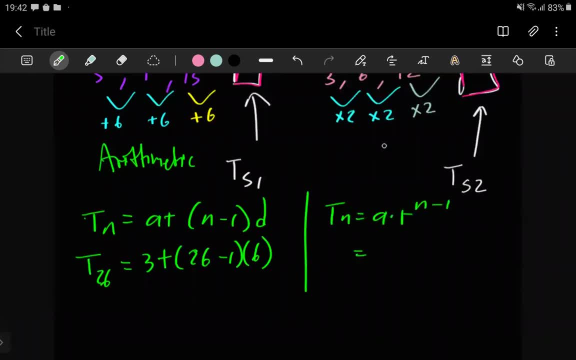 geometric. we do the same for the geometric. But we do the same for the geometric. We do the same, for we use the formula for a geometric sequence: A- here is a three, R- we see it's a two, N is 26.. 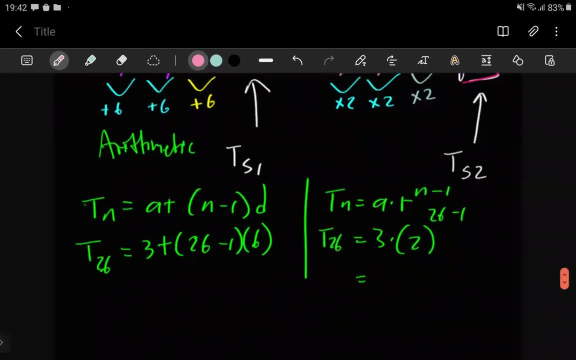 So T26, and then here let's see T26. And then let us put all this into the calculator- And I'm thinking where in the values may calculate just like your. it is so far, So let me just try and do this quickly. 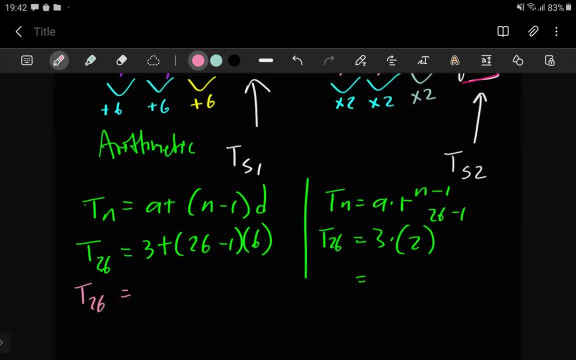 So it's like 25 times six plus three. I'm getting 153 here, So let's put here 153.. And then here you're not. this one is gonna be a bit tricky. What is two to the power of 25?? 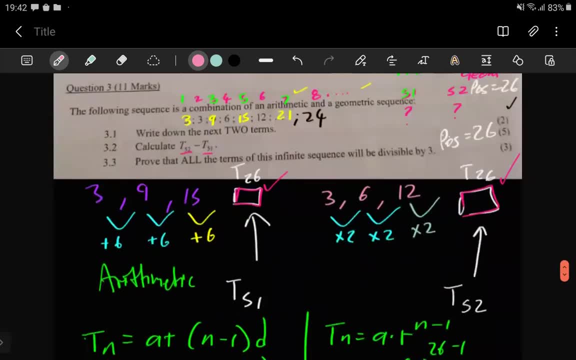 Yup, this one is super tricky. Let me just get a calculator so that we can do what we need to do. Calculator- where are you? I hope I haven't lost my calculator, or there it is. There, it is, I found it. 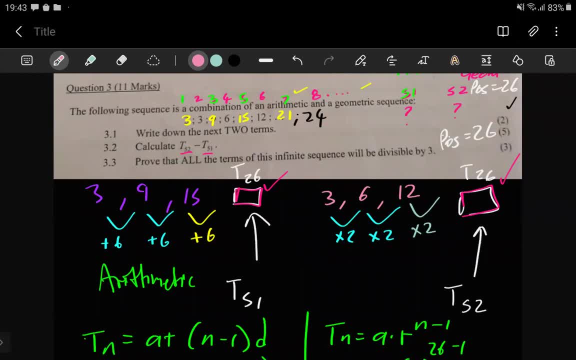 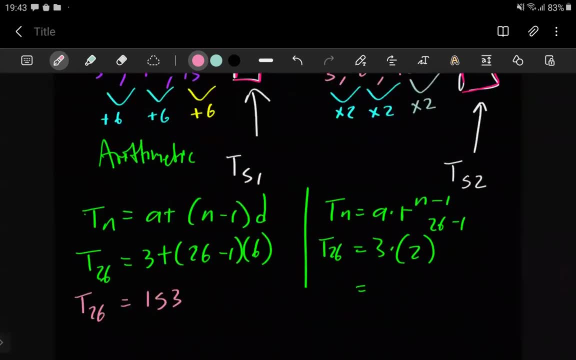 Okay, yeah, So in the second equation. in the second equation, let's see here This is: oh, so that? sorry, I moved away from someone that needs to be hearing me. So in the second equation, it's just two to the power of 26. 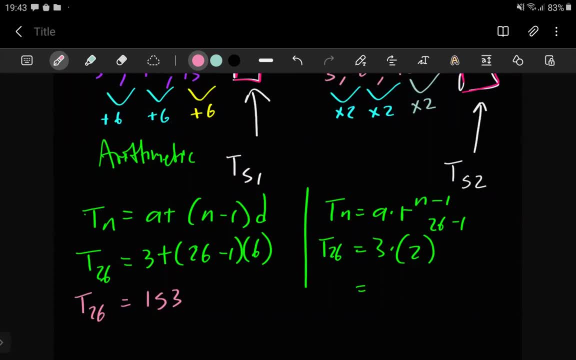 minus one and then multiply that by three, Yo, that's a huge number. like goodness, Goodness, yes, yes, like this number looks illegal, but then is: let's just do it again so that we can make sure that we definitely have the correct number. so it's a huge number for the second one, right? 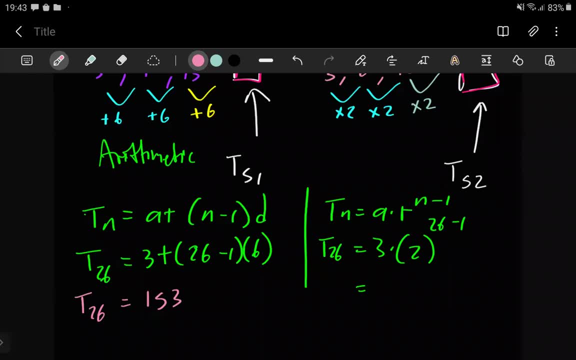 it's like: what is it? well, i'll just write it out and then i'll say it. just now, it's like one here, zero, zero, six, six, and then there's like three there, two, nine, six, two, nine, six, wow, what a wow. anyways, let's see, this is like three, three. so this is like a hundred million, six hundred, and 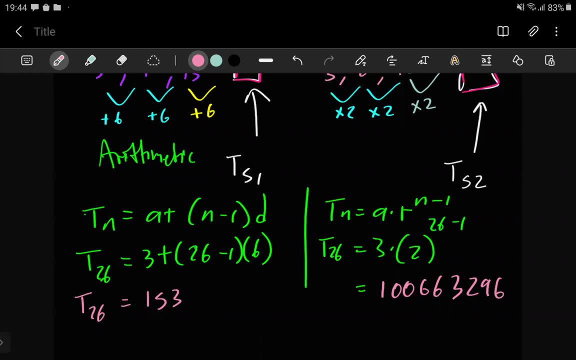 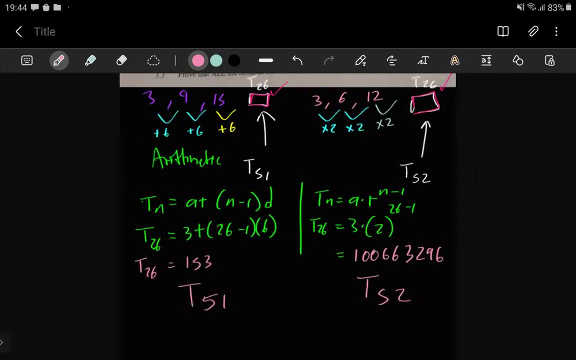 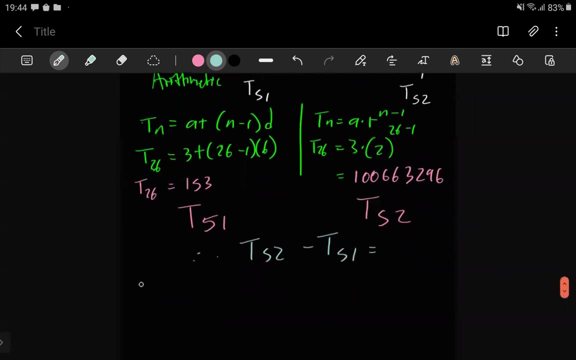 sixty three thousand two hundred and ninety six. okay, so clearly, this is t 52, this is t 51, like we said. so we already know that, therefore, t 52 minus t 51 is going to be equal to one zero, zero, six, three, two, nine, six minus.